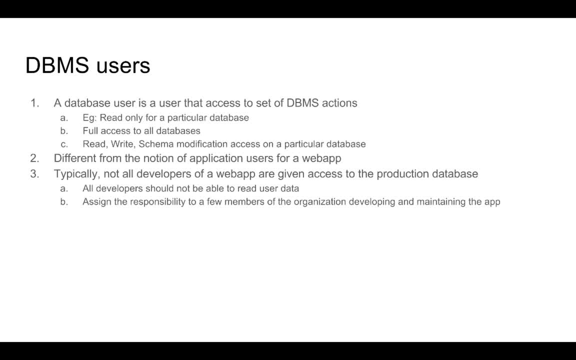 actions, For example, in the practical modules that we did last week. when you went to the IMAT console and clicked on create DB credentials, a user name and a password was generated that allowed you to access a specific database. The database was also named after the user. 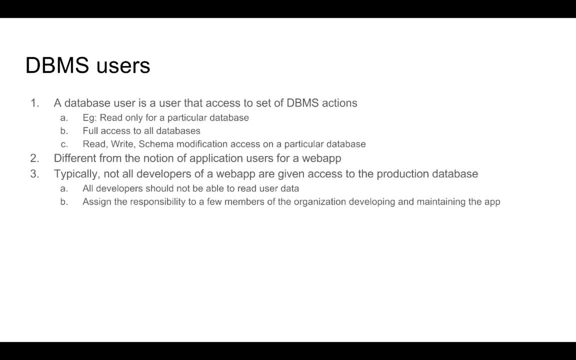 name. So permissions to create data, to modify schema inside the database, to update data, to create indexes, to update indexes, etcetera, were all privileges that were given to that user on that particular database only. Similarly, you can actually create more users, have more. 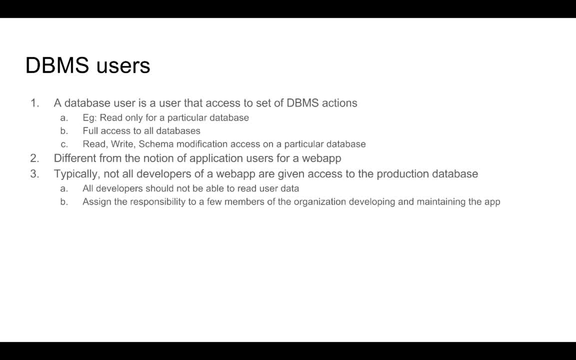 specific privileges on one or more databases. It is important to understand that when you are creating a database, you need to have to understand that a database user is very different from the notion of an application user for the web app, For example. in my case I use the user name coco98 to login to a database. 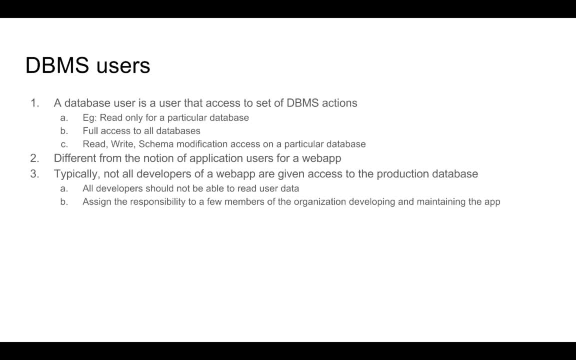 called coco98 and perform actions there. However, in my database I had the data models for the user table and the articles table, and the user table contained users that had nothing to do with the user coco98. So application users are different from database users. The 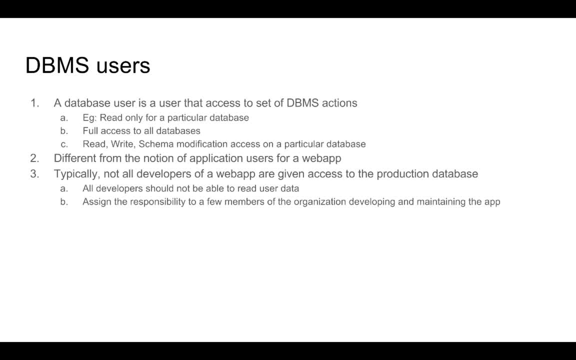 reason why database users are an important concept is that they are different from the user table. The reason why database users are an important concept is that they are different from the user table. The reason why database users are an important concept provided by most mature DBMS systems today is because typically in an application, not 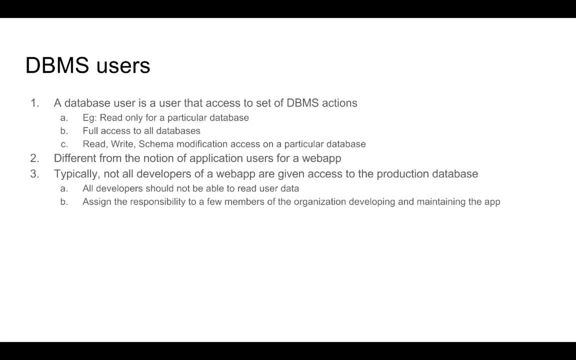 all developers are given access to the production database. Only a few key members of your organization will have the access to the database credentials, which will allow your web app code to talk to your database. So the way to ensure appropriate security of your databases that are managed. 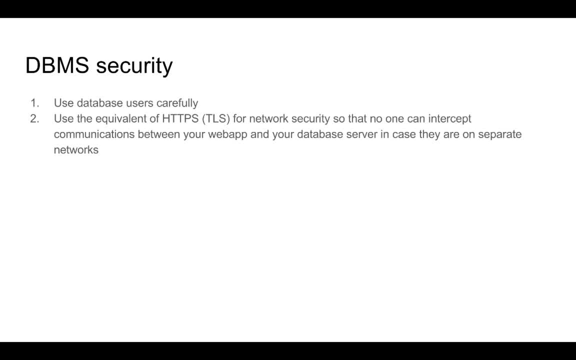 by your DBMS is to use database users carefully, So we should create appropriate roles for members within our organizations and appropriate access credentials for the different pieces of software that access the database. We should also use the equivalent of HTTPS, which is called TLS for network level security, so that nobody can intercept the connections. 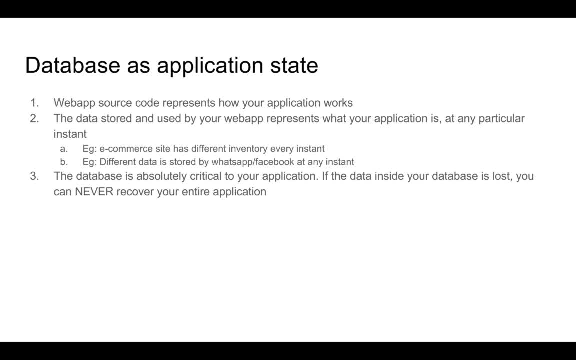 between the web app and the database server. Now the database is essentially the state of the entire application. The web app source code of our application represents how the application works, but the database actually represents what the application is at any particular instance. The e-commerce site has a different amount of stock at any instance, So what the state? 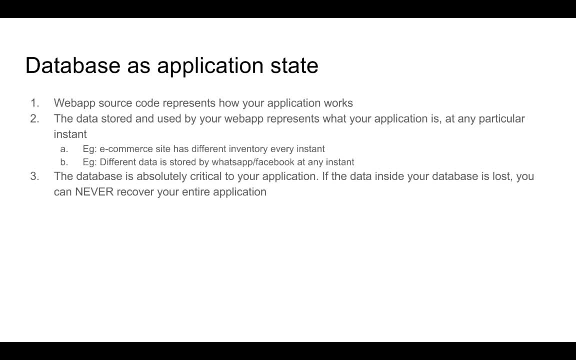 of the e-commerce site is represented only by its database. If we lose the information inside the database, our entire application actually cannot be recovered. In case we lose portions of our source code, it might be possible for us to recover our source code or to rewrite. 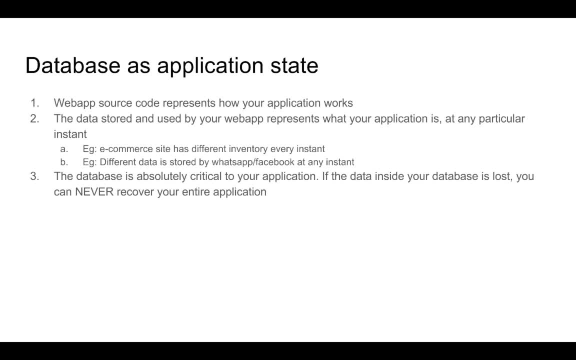 our source code, but in case data that has been dynamically created by the activities of our web app or the activities of our users are lost, the entire state of the application as it was. So it is extremely important to start backing up our database, and every DBMS provides several. 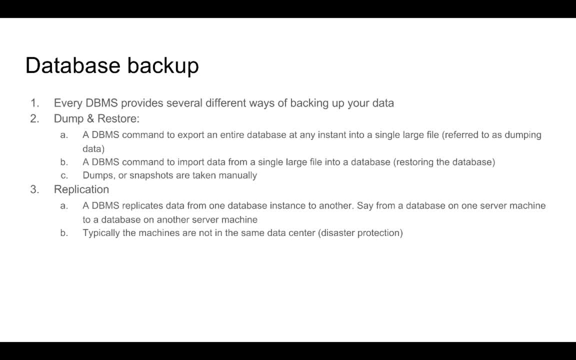 different ways of backing up data. The most common method is dumping and restoring data. So DBMS has provided commands to export an entire database into a single file or into a set of single files, and this is referred to as dumping data. Another DBS command allows: 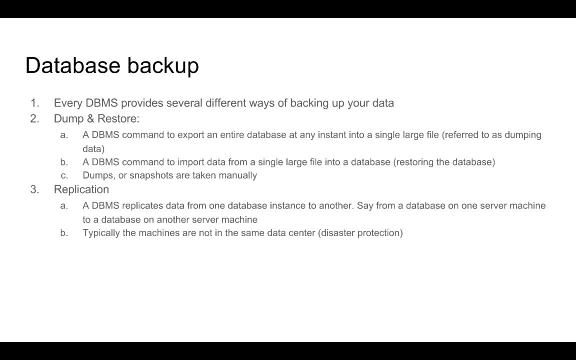 to import this set of files or a single file and use that to create or populate an existing database. So we can take dumps or take snapshots of the database manually at regular intervals and then, in case of emergency situation when a restore is required, the database is restored. 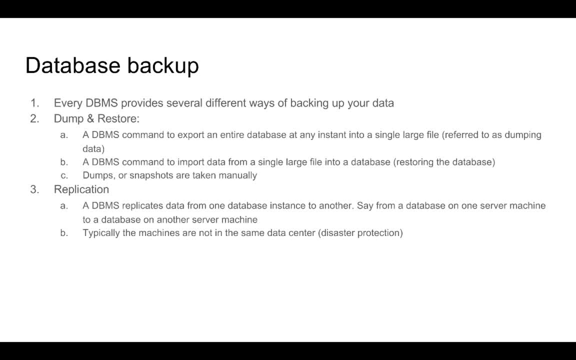 from this dump or from this snapshot. This obviously means that the last state of the application that we have is when the snapshot was taken and all the information that was captured in the database after the snapshot was taken is lost. Another style of backup which is more automated is replication. DBMS replicates data from one 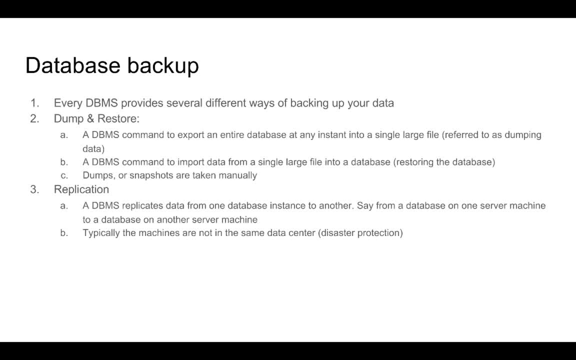 database instance to another. Say we have one instance of a DBMS which has a database on one server machine and another DBMS with another database instance on other server machine. Modern DBMS allow a particular configuration that allows data to be replicated from one database to another. So typically these machines are also not kept in the same data center. 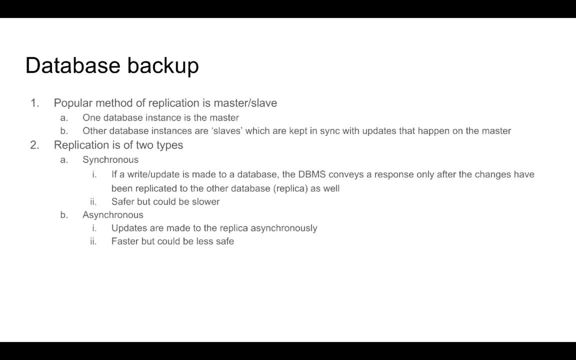 for a disaster protection. A popular method of replication is master-slave. One database instance is called the master and the other database instance is called a slave, So slaves. These are kept in sync with updates that happen on the master. all the activity happens on. 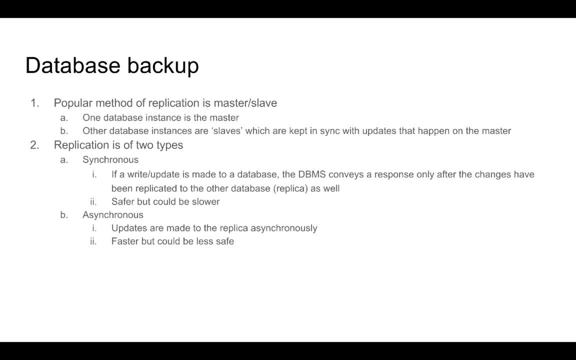 the master database. So the web app communicates with the master database and all of these updates are propagated to the slave databases. So now, in case something goes wrong on the master database, we can always recover from the slave. This is the advantage: that, in case something goes wrong, we can recover our data. we can. 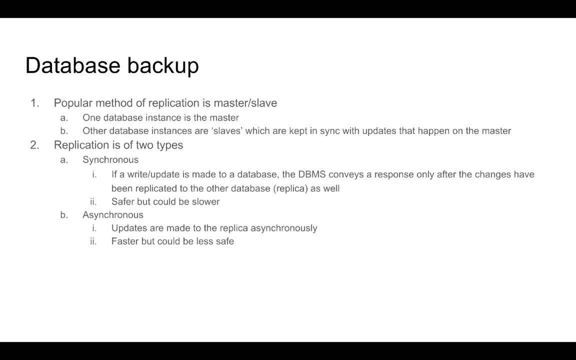 recover almost all of our data from the slave replica of our database. There are two kinds of replication. there is synchronous and asynchronous replication. Asynchronous replication is when updates are transmitted from the master to a slave, and only once the updates have actually been propagated to the slave as well does the 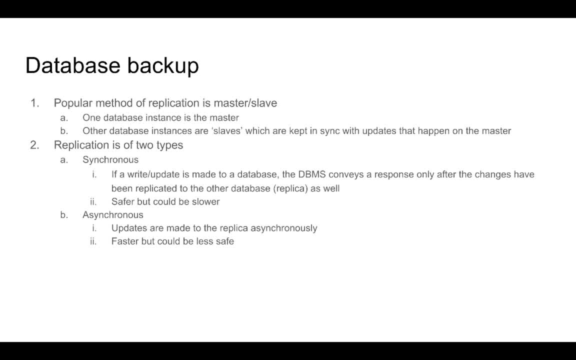 master actually say that an update has been committed. So this is a very safe method of replication, but it can be slower because we are not just updating one database. every time we update with the master, we are updating the master and the slave database. 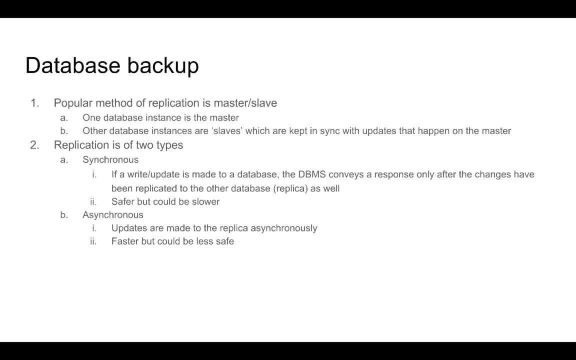 Asynchronous replication is when updates are made to the master but the master does not wait to propagate those updates to the slave replica. The master responds immediately. So updates to the slave replica are made asynchronously. This is faster because the master database responds to updates much faster, but it is 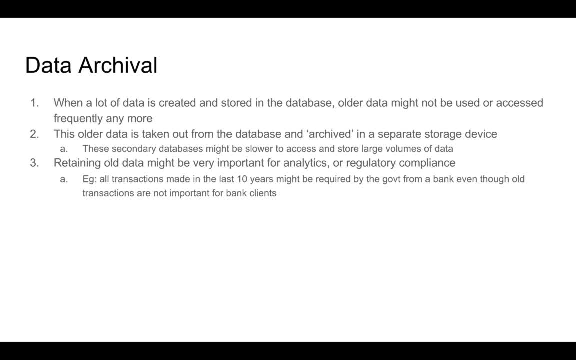 potentially less safe than synchronous replication. Another concept is the concept of data archival. In applications where a lot of data is created, some of the older data might not be very useful or might not be accessed very often. In this case, old data is actually taken out from the database and archived in a separate. 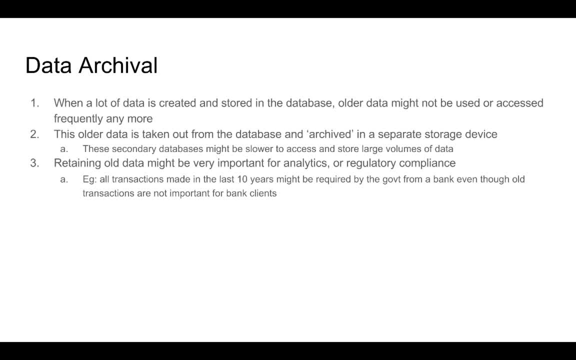 storage device. These secondary databases actually might be different kinds of databases. They might be on different kinds of hardware that are slower to access and are able to store larger volumes of data. It is important to archive this old data and not just delete the old data, because the old 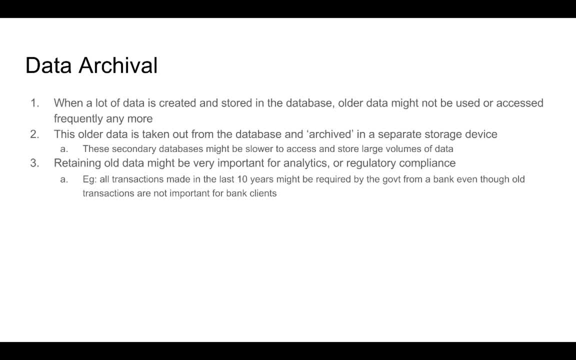 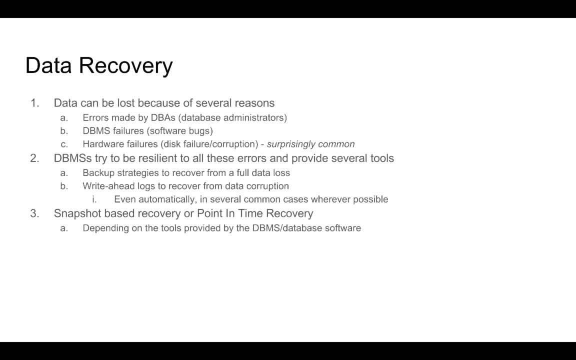 data might be important for analytics purposes or for regulatory compliance purposes. It is important to think about data recovery and what kind of guarantees we want for the data recovery of our application from the very beginning. It is important to think about because data can be lost because of several reasons. 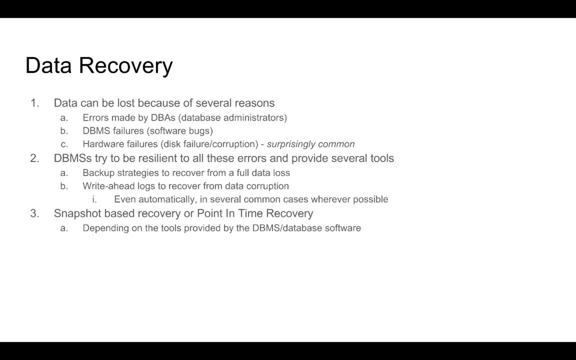 Errors can be made by database administrators. There might be software errors in the DBMS. There might be hardware failures where the disk fails or there is disk corruption. This is actually a surprisingly common failure. To be resilient to these kinds of errors, it is important to think about what the recovery. 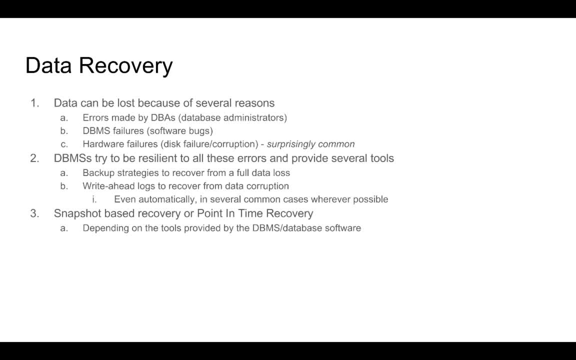 characteristics of our applications are: How much time do we want to be able to recover our entire database and our application when our application is live? Most DBMSs try to be resilient, fairly automatically, to most of these errors. For example, we discussed that. 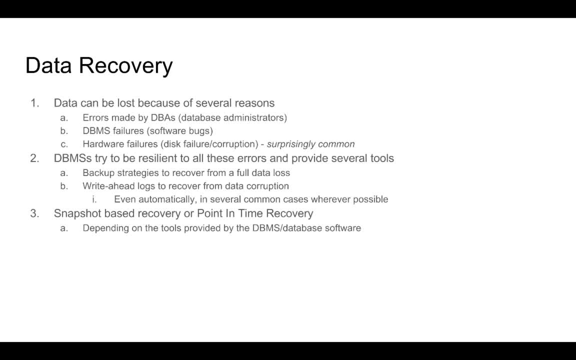 Most DBMSs try to be resilient to most of these errors. Most DBMSs provide backup strategies that allow a recovery from full data loss, but in case there is partial data corruption, then databases try to recover from it automatically, like we discussed transactions in the last module. 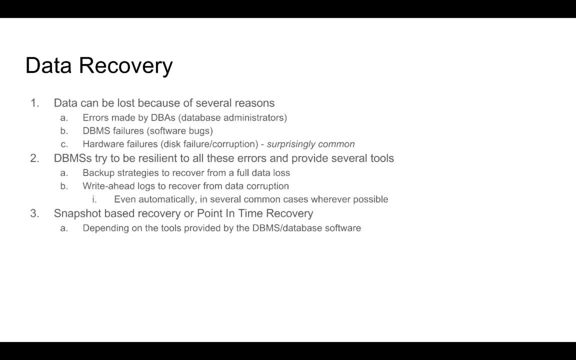 In case a transaction could not complete entirely, the database detects that a few operations have happened which need to be rolled back, and the database is able to roll back those operations. Databases like Postgres use the concept of a write ahead log. A write ahead log is essentially a log. 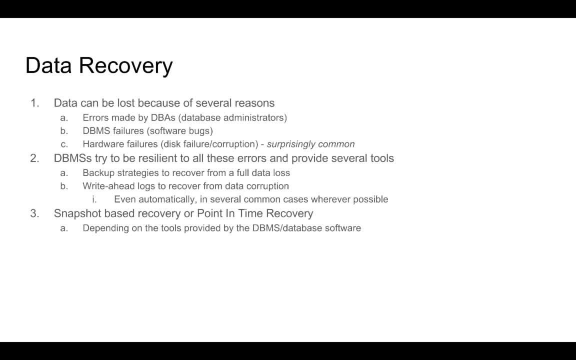 A write ahead log that is maintained by the DBMS logs all the actions and queries that are made by users into a file and once the query is logged into the file, the database server actually applies that query on to the database. This is the advantage that in case something goes wrong, that in case the query has not, 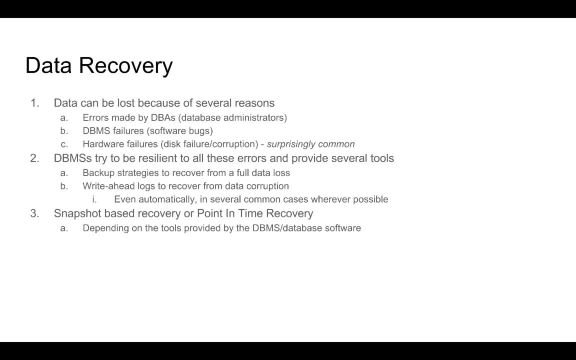 been completely processed and applied to the database. the database server can read the write ahead log to figure out what the query was and replay the query. Another style of data recovery is called pre-recovery. Pre-recovery is a type of data recovery. 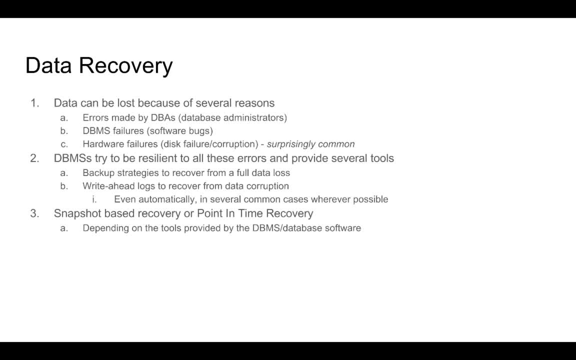 It is called point in time recovery. When we discussed the data backup strategy of dumping and restoring, we were looking at what is called snapshot based recovery, where we were recovering a snapshot of the data from the time the database dump was taken. A point in time recovery is a more complex kind of recovery when we want to recover the 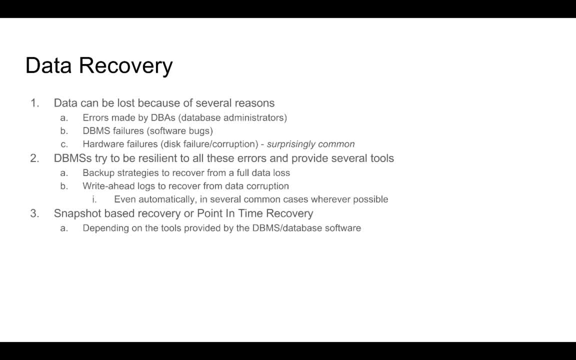 database state as it was at any particular time in the past. So a point in time recovery method allows us to choose any particular moment from the past. We can move through all those different queries as they executed and choose an exact particular instant at which we want to reset our database, and this can be done only by specialized tools. 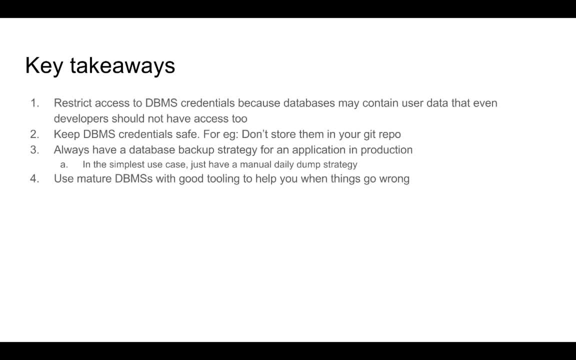 that are provided by specific DBMS and database softwares. The important things to take out of this short module are: number one: we should be very careful about the database credentials that we generate. If we are not careful about these database credentials, then people will have access. 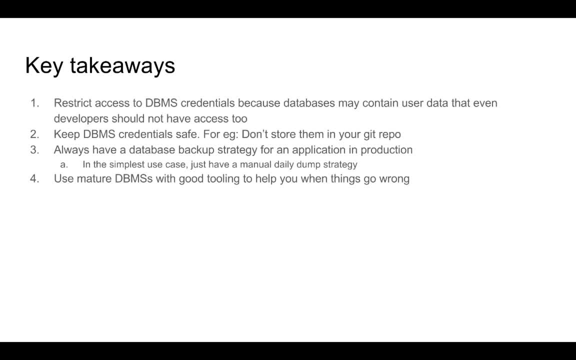 to user data that is stored in the database. It is important to keep these DBMS credentials. For example, these credentials should never be stored in a git repository because in case it is an open source project or if the project source code is open, then people can just.